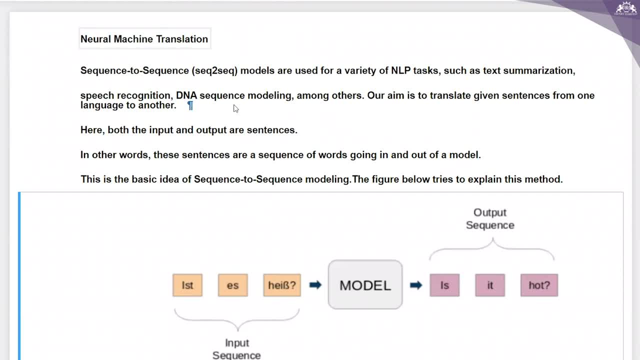 over here We are trying to convert German language into English. That is why it is called as machine translation. So the model, what I am going to use over here, is sequence to sequence model. So these sequence to sequence models are used on variety of NLP tasks, like text summarization. 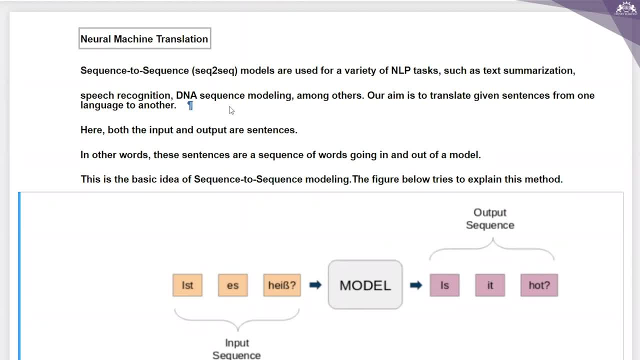 speech recognition, DNA sequence modeling, and there are many more applications. So here, what is our objective? over here? We are trying to convert one from one language to another language over here. So what are we trying to do? We are trying to translate some sentences from one language. 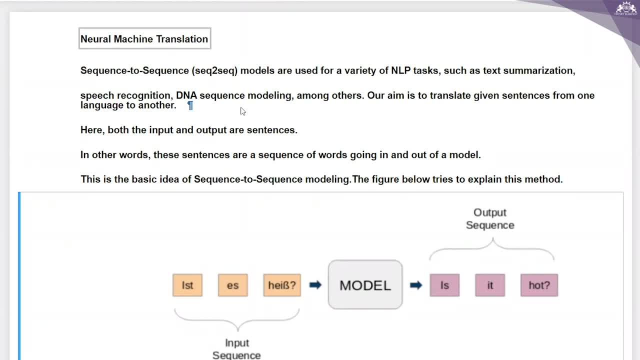 to another language. So what is input and output over here? Both are going to be the sentence, So the input sentence is going to be German language and the output sentence is going to be an English. So in other words, these sentences are a sequence of words. 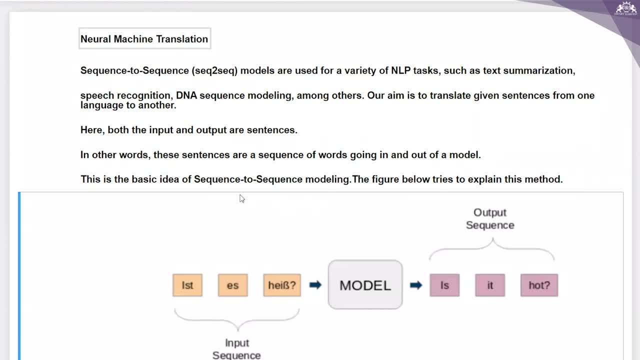 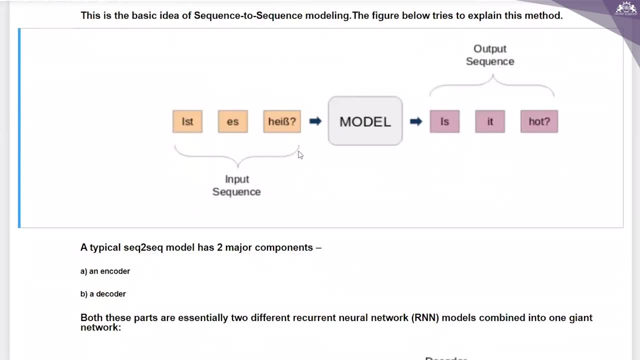 going in and out of a model. So this is the basic idea of sequence to sequence modeling. So now let us try to understand. So this is basically the input sentence that is being in German and I am using the model and the output. I am getting it in English. I do not know German. 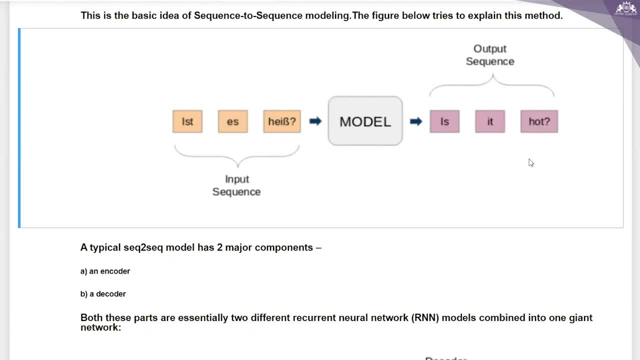 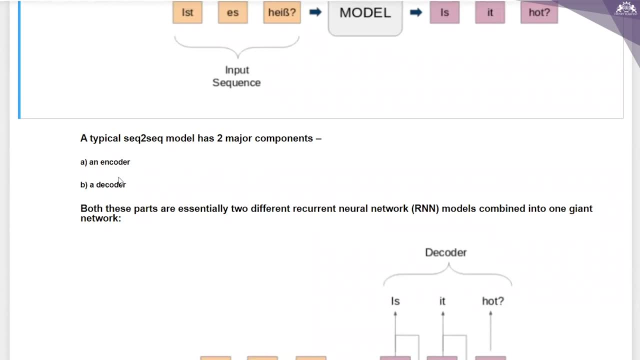 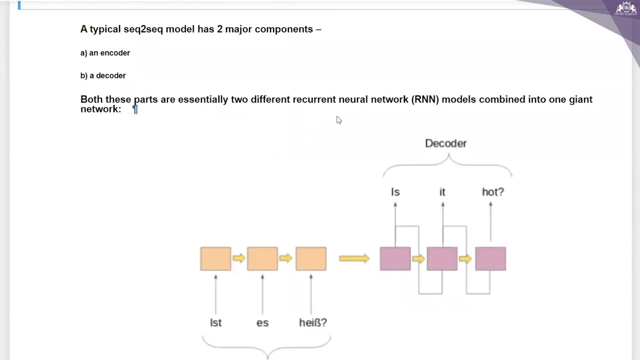 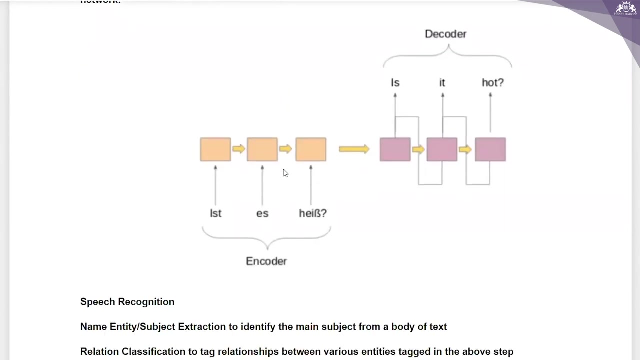 but still the meaning of it is: is it hard? So a typical sentence, sequence to sequence model, has two components: One is an encoder and the other one is decoder. So both encoder and decoder are two different recurrent neural network models combined into one giant network. So you can see over here this is basically the encoder and this is the decoder. 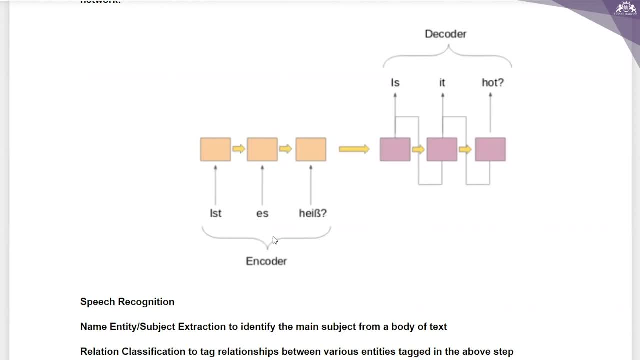 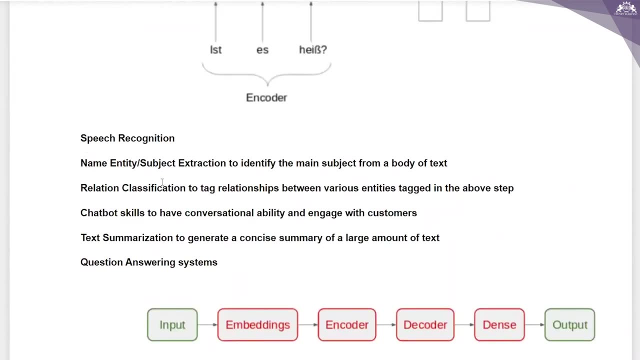 Right. So there are several use cases. So let me give you some examples, like speech recognition, named entity recognition, subject extraction to identify the main object from a body of text, Then relation classification to tag, relationships between various entities tagged in the above step. 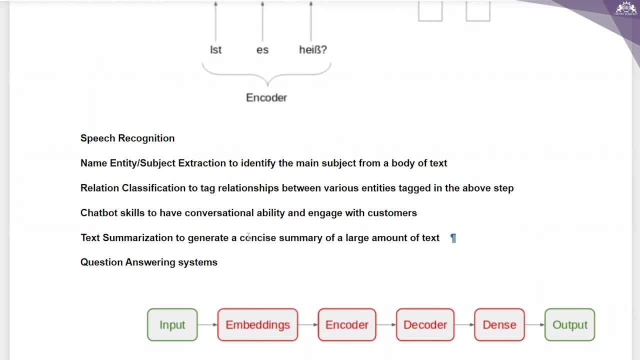 And chatbot skills to have conversational ability and engage with customers. Text summarization, text summarization And, finally, text summarization To generate a concise summary of a large amount of text. And the last one is question answering systems. So what we are going to do is we are going to implement in Python, using Keras. 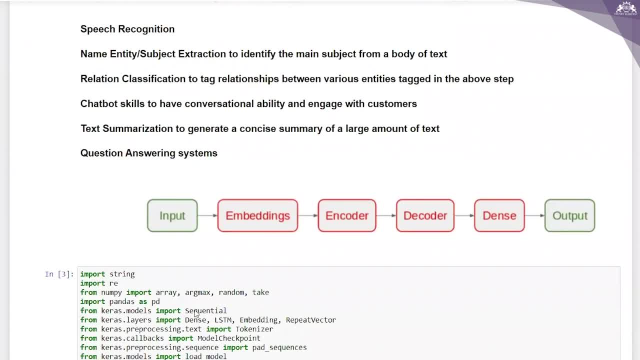 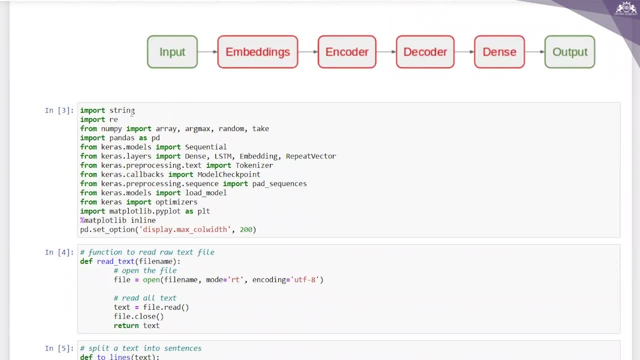 Right, Fine. So let us try to import all the required libraries. So import string import re. So import string import re From numpy import array argmax random. take import pandas as pd And from kerasmodels I'm importing sequential. 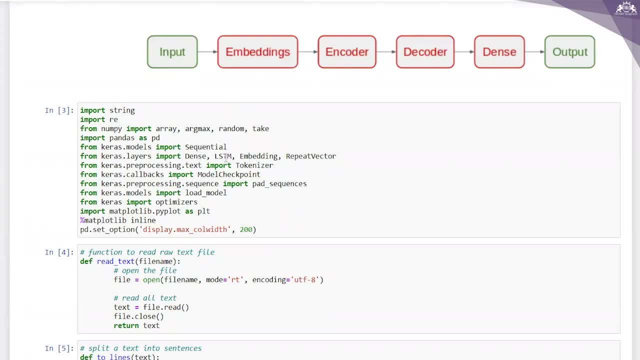 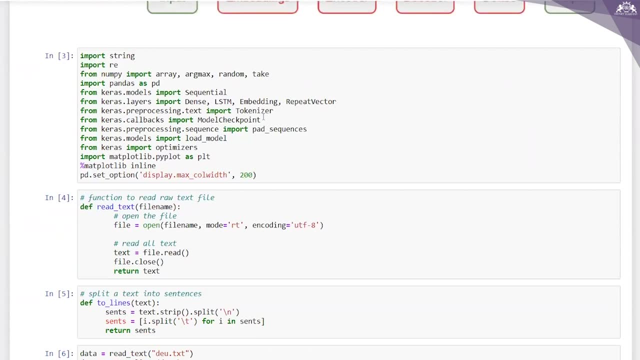 From keraslayers. I'm importing dense lstm embedding repeat vector And from keraspreprocessingtext I'm importing tokenizer From kerascallbacks. I'm importing model checkpoint From keraspreprocessingsequence. importing tokenizer pad underscore sequences from keras dot models. import load underscore model from keras import. 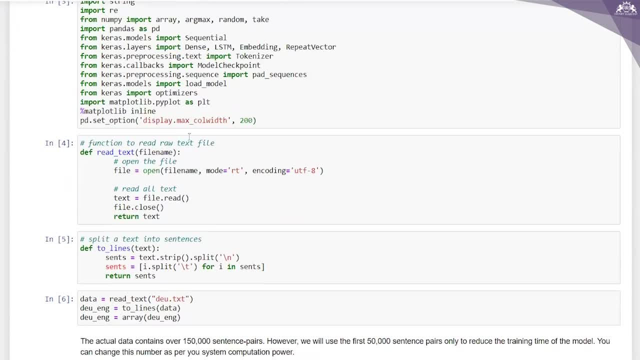 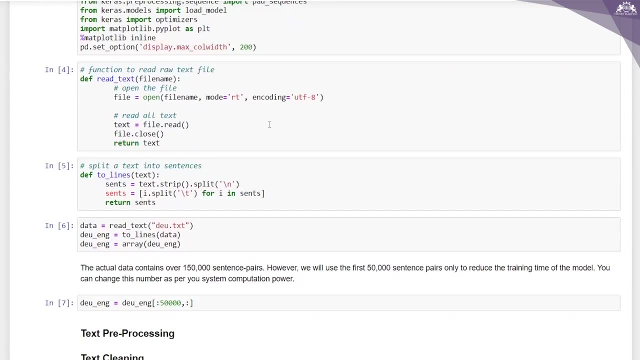 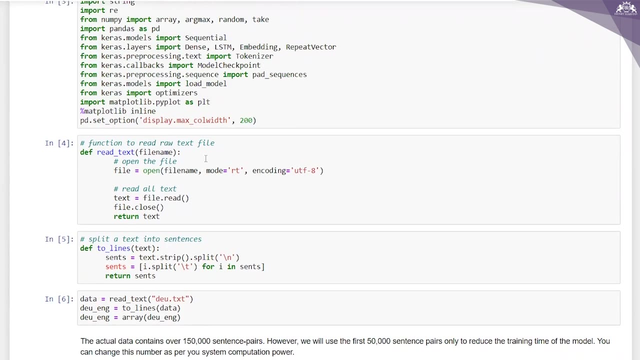 optimizers: import matplotlib. and then i'm just setting the option for display max call with column width as 200, right? so this is being done. what is the next step? we have to read the data into our ide, right? so this is basically a text file of english to german sentence pairs, right? 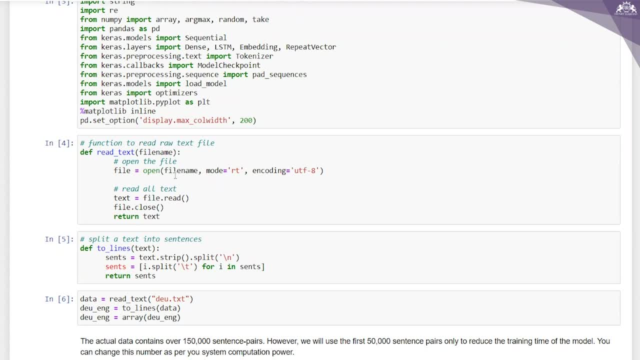 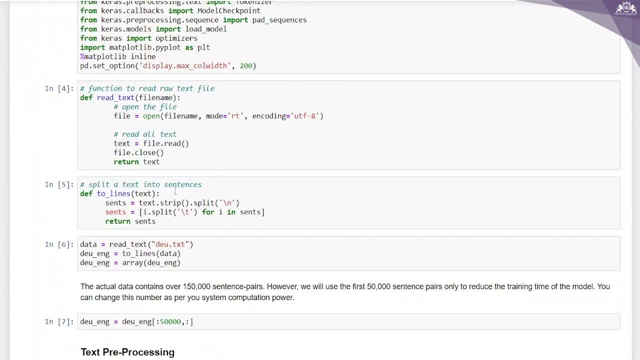 and first we will read the file using a function defined below. so i'm using this code for the function to read raw text file, right? so let's define another function to split text into english, german pairs separated by this. so we will then split these pairs into english sentences and german sentences respectively. 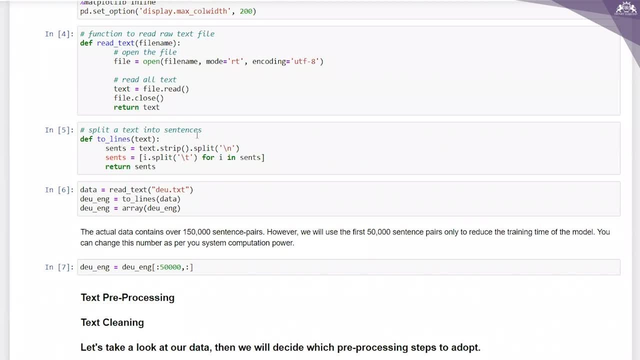 right. so what i'm doing? i'm splitting a text into sentences. now we can use these functions to read the text into an array in the desired format. right, so now. the actual data contains over 1 lakh 50 000 sentence pairs. however, we will use only the first 50 000. 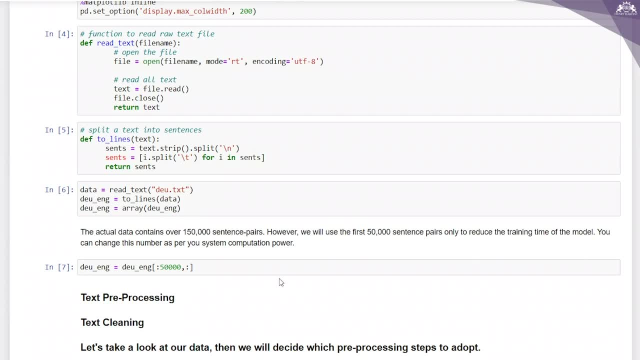 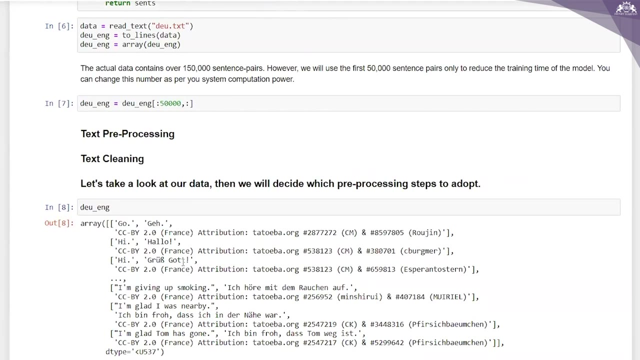 000 sentence space only to reduce the training time of the model. so, in case, if you want to change the number, in case if you want to train on 1.5 lakh sentence space, you can do that, but i have taken only the first 50 000 right. what is the next step? the next step? so i have imported all the 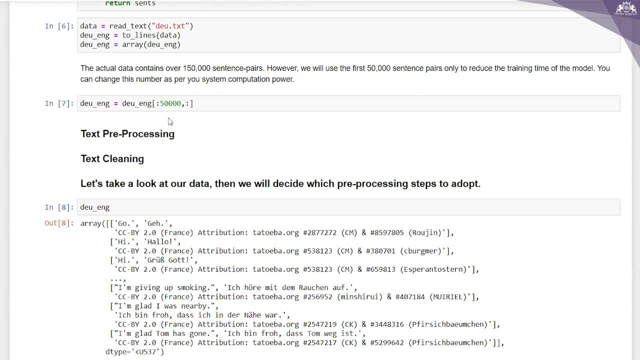 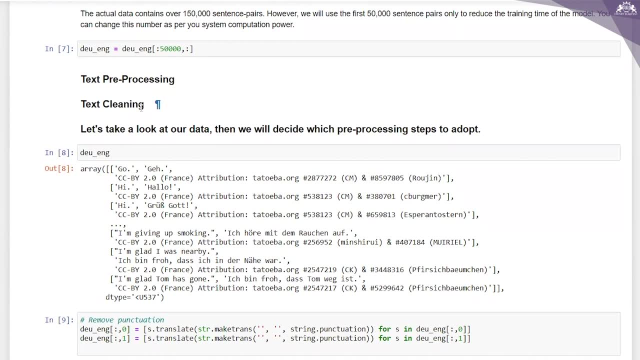 necessary packages and the second step. i have loaded the data right, so now i have to start with the text pre-processing. so basically it is nothing but the text cleaning step i'm going to start with. so there is an important step in any project, uh, so that is especially in nlp. so the 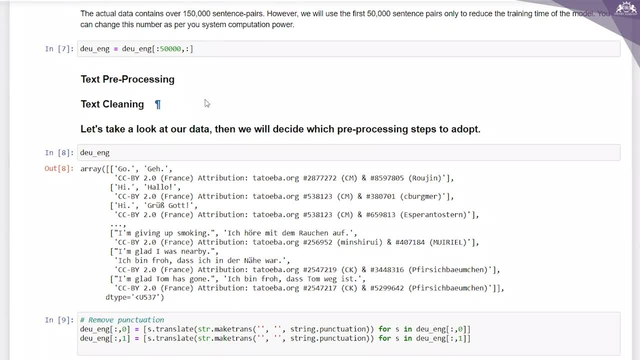 data. what we are going to work with is basically the unstructured data, so there are certain things we have to take care before jumping to the model. so the first step, what i'm going to do is text cleaning. so just look at our data, then we will decide which pre-processing steps have to be. 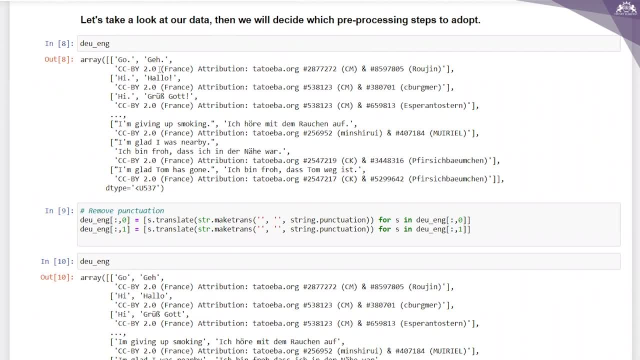 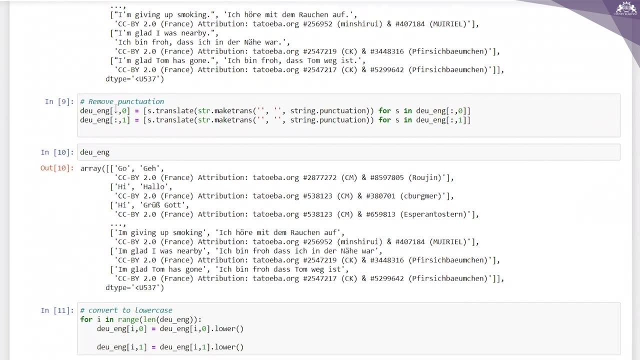 adopted, right? so de you underscore english and then this is the array output i'm getting over here. so we will get rid of all the punctuation marks and then we can convert all the text to the lower case, right? so that is what i have done: remove punctuation. 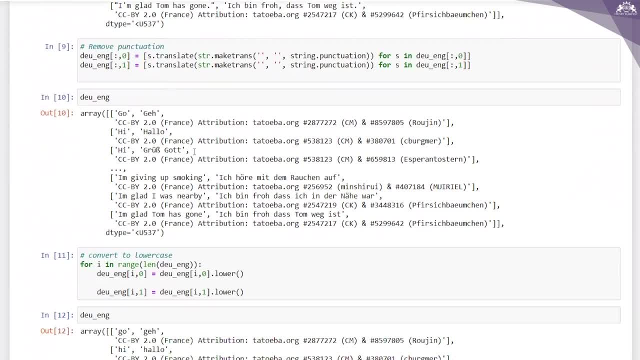 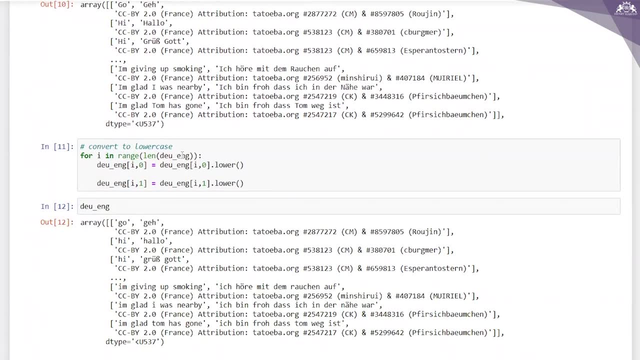 so, basically, i'm trying to remove all the punctuation. so this is the output i'm getting now, and then i'm trying to convert it into lower case, right? so once i do that here i have done two steps. one is about, uh, removing the punctuation and then converting. 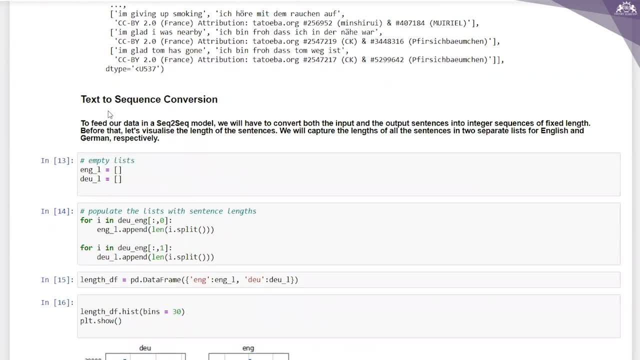 to the lower case. what is the next step? i'm going to do text to sequence conversion, right? so a sequence to model requires that we convert both the input and output sentences into integer sequences of fixed length and length. so, but before we do that, we have to visualize the 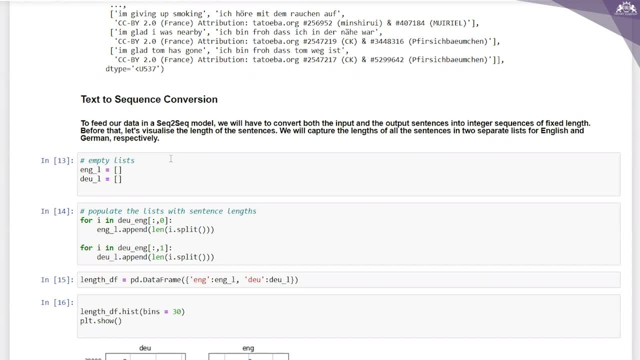 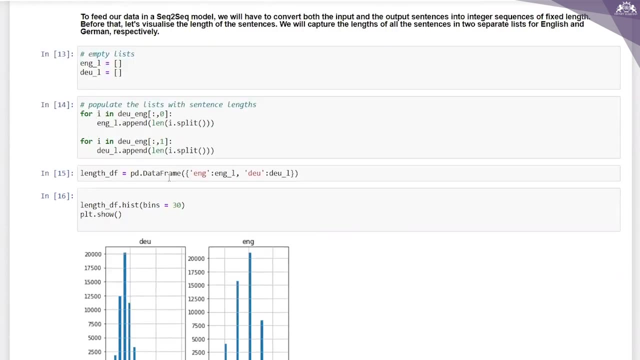 length of the sentences, right? so we have to capture the length of all these sentences in the two separate lists for english as well as the german respectively, right? so this is what we are trying to do now. so, quite intuitive: the maximum length of the german sentences we will. 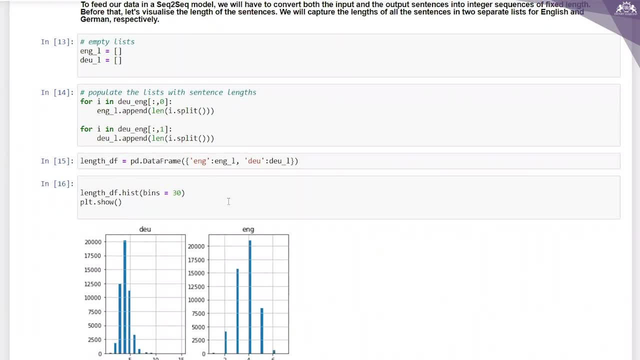 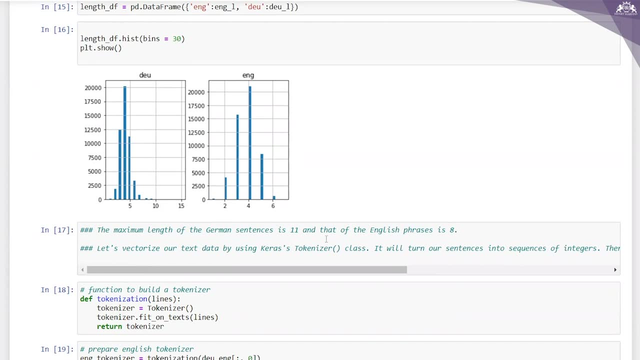 uh, try to figure out, right. so this is what we have to try to figure out. so what i identified is the maximum length of the german sentences is basically 11 and the english phrases is 8, right? so let's vectorize our text data by using the. 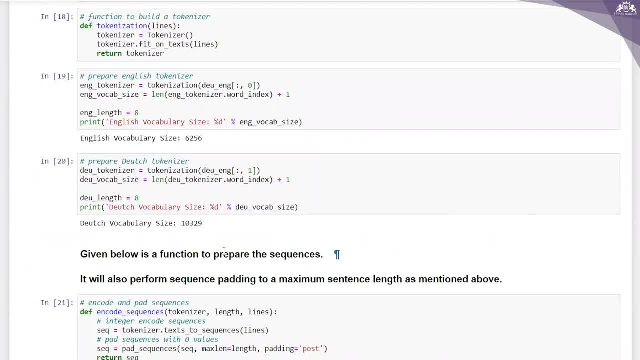 keras tokenizer, right, fine. so now i have defined a function to build a tokenizer. so what will happen now? it will turn our sentences into sequences of integers. then we can pad those sequences with the zeros, right. we can pad those sequences with the zeros to make all the sequences of the same length, right. so we will prepare the tokenizers for both. 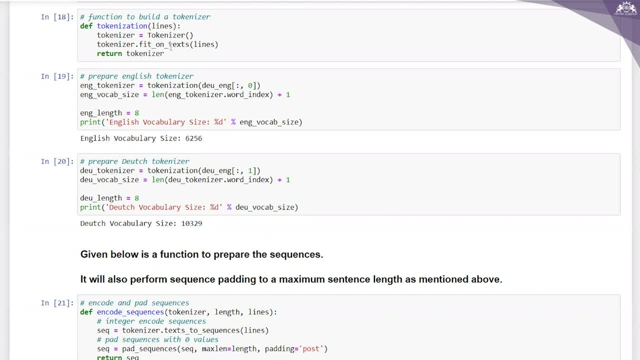 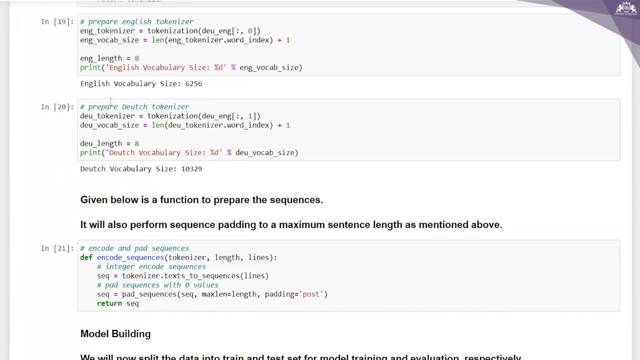 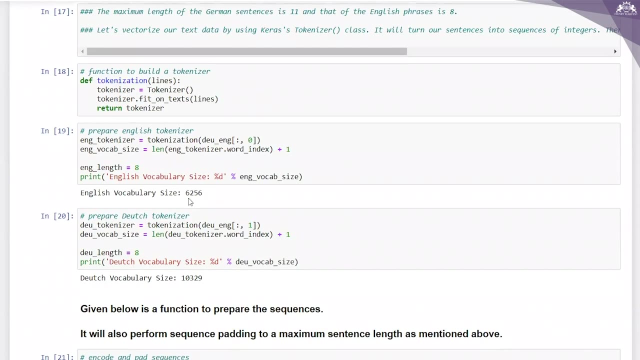 german and english sentences right. so this is what i have done. uh, so a function to build a tokenizer and then i am preparing english tokenizer and this definition tokenizer right. so once i do that, so just i'm trying to get the vocabulary size of english that i'm getting it as 6256. 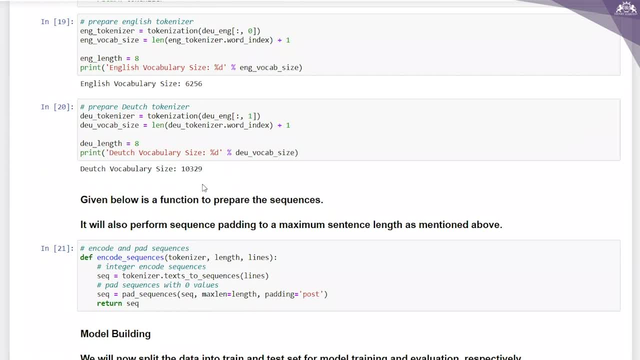 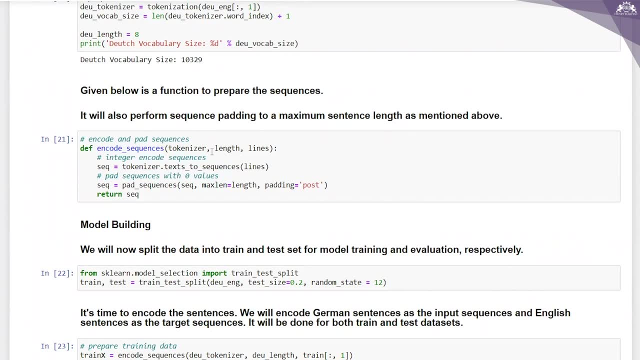 i'm getting it as 6256. i'm getting it as 6256 and this german, i'm getting it as 10 329. right, so now? uh, this is the function to prepare the sequences. it will also perform sequence padding to a maximum length, as i mentioned above, right. 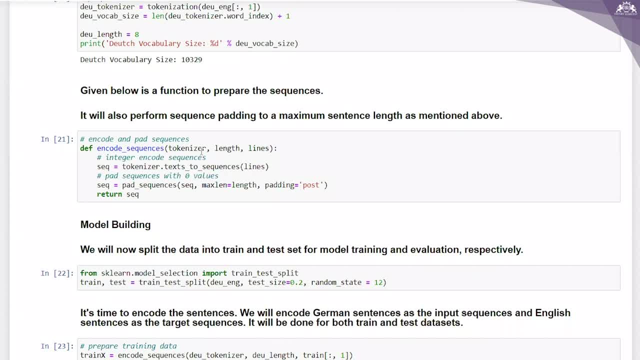 so now there will be a block that contains a function to prepare the sequences, so it will also perform sequence padding to a maximum sentence length, right? so this is what we are going to do: encode and pad sequences. so define, encode sequences, tokenizer length, as well as the lines, and then i am writing integer: encode. 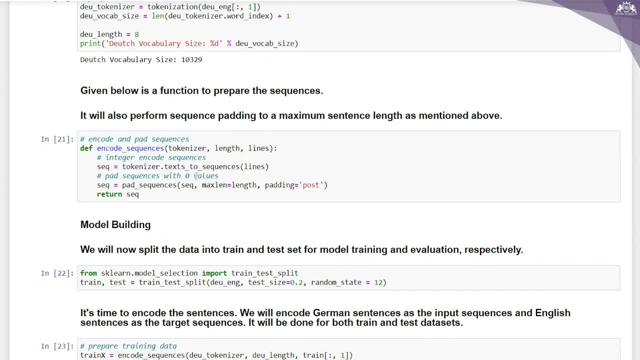 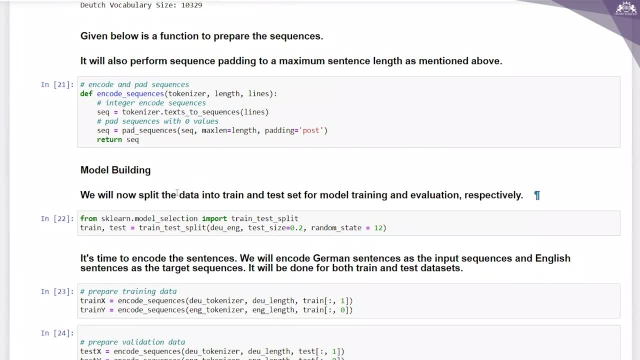 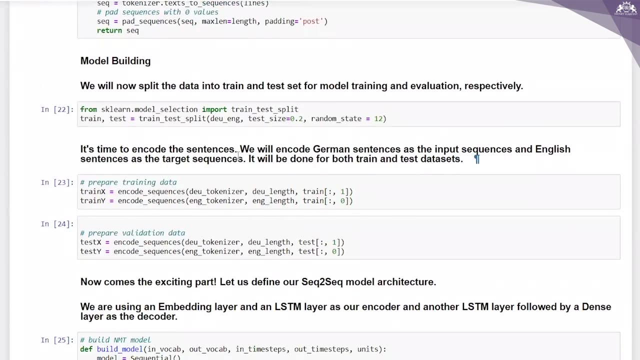 sequences and then padding sequences with the zero values, right. so now everything is being done. now we can start with the model building. so while we build the model, we have to split the data into train and test set for model training and evaluation. so from sql on dot model underscore selection, import train underscore, test underscore split and 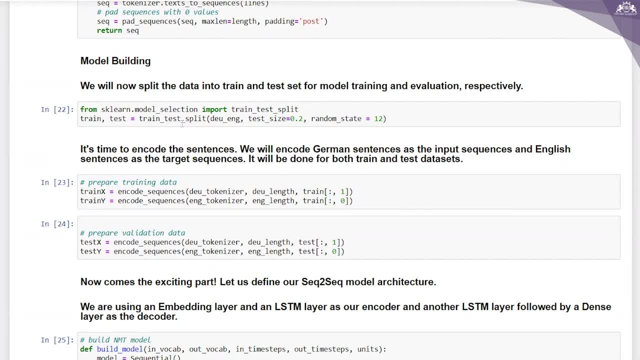 then train underscore test is equal to train underscore test. underscore split that i have imported and this one i'm writing. test sizes point to random underscore state and giving it as 12. you can change all these numbers and see right. so now it is time to encode these sentences, so we will. 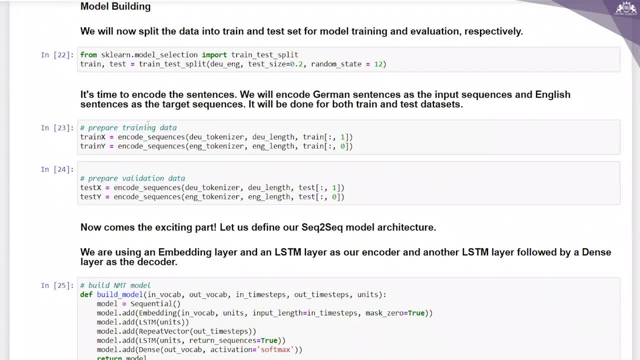 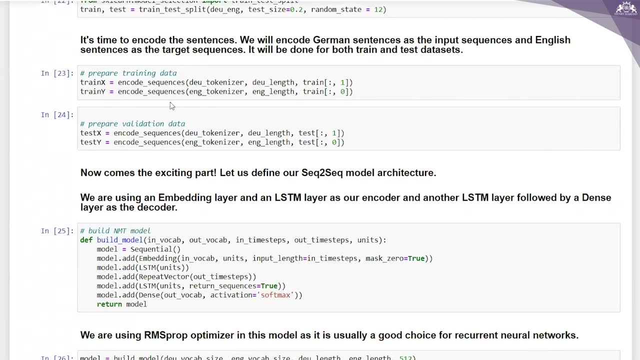 encode german sentences as the input sentences and english sentences as the targetter. why? because we are trying to convert german into english, right? so it will be done on both the training set as well as the test data set. now i am preparing with the training data, so i am encoding the sequences. 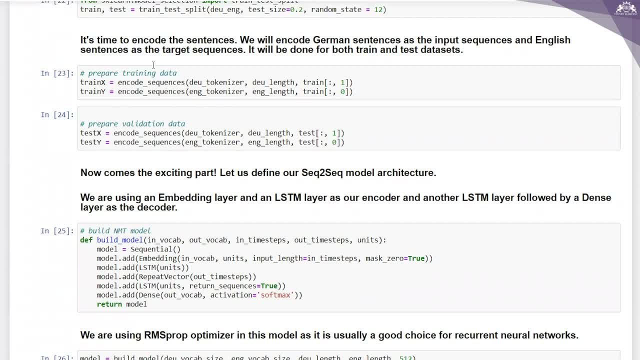 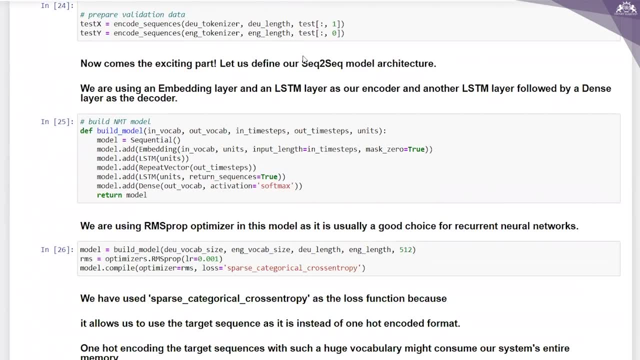 and this is what i am passing it now, and then actually, i'm preparing the training data as well as the validation data. right now- this is the super cool part- we are going to define our sequence to sequence model architecture, so we are using an embedding layer and an lstm layer as the encoder. 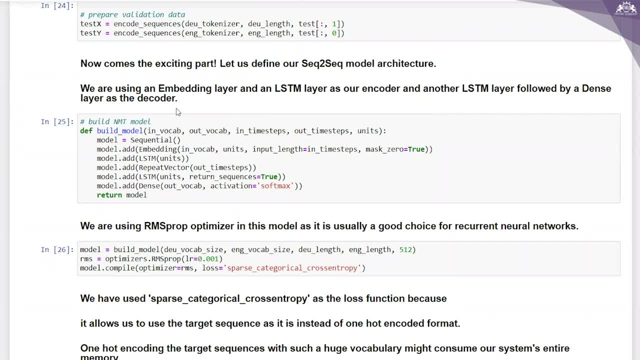 and another lstm layer followed by an dense layer as the decoder. so you can see, over here i am building neural machine translation model now. so i'm building the model and here i'm passing these arguments in underscore vocabulary out, underscore vocabulary, in underscore time step out, underscore time steps and units and model what. 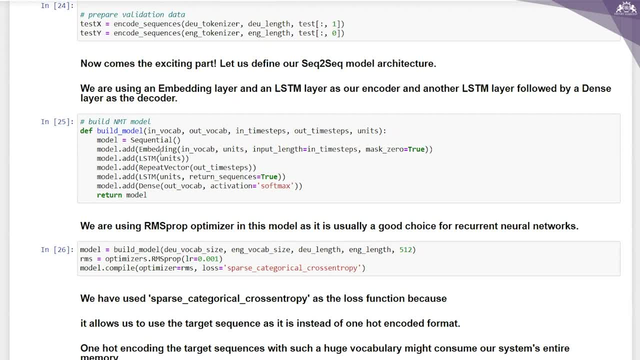 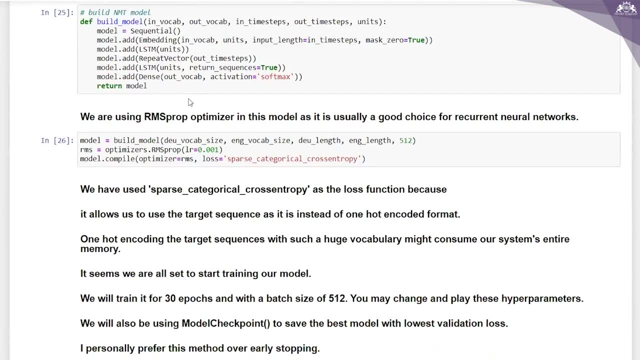 i'm using. i'm using sequential. now i'm adding embedding. i'm adding lstm. i'm adding repeat vector. i'm adding again lstm. again i'm adding denser. so in the dense i'm using activation function as softmax. i'm returning the model. so now we are using: uh, okay, so now, uh, what we are using. 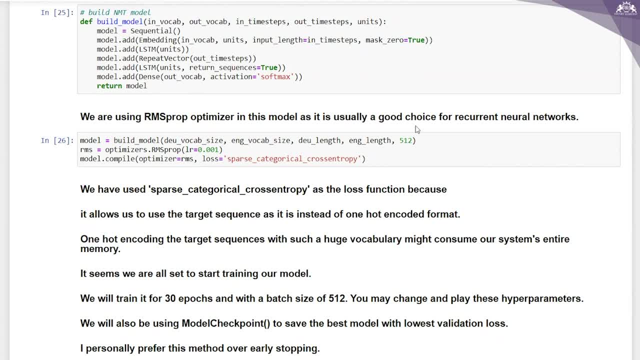 is rms prop optimizer, uh, as, because it is a good choice for recurrent neural networks. so i'm just building the model. i'm i'm just building the model. uh do vocabulary size. english underscore vocabulary size. new underscore length: uh and english underscore length that is 512. i have taken. 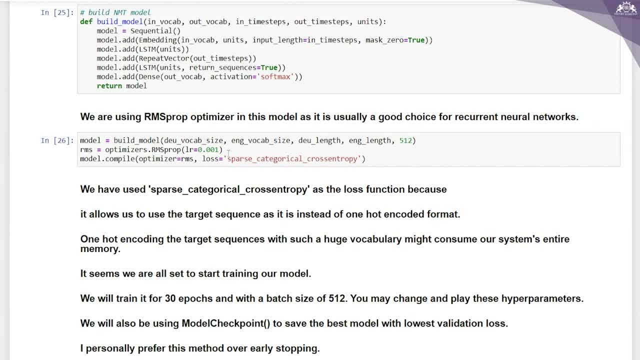 and then rms prop learning rate and specifying it as 0.001, and then i'm compiling the model optimizer. what i am using is rms loss. i am using it as sparse underscore, categorical underscore, cross entropy, right. so this is what i have. uh, this is what i have done. 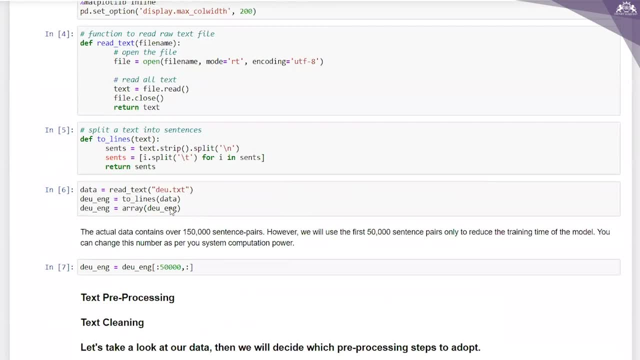 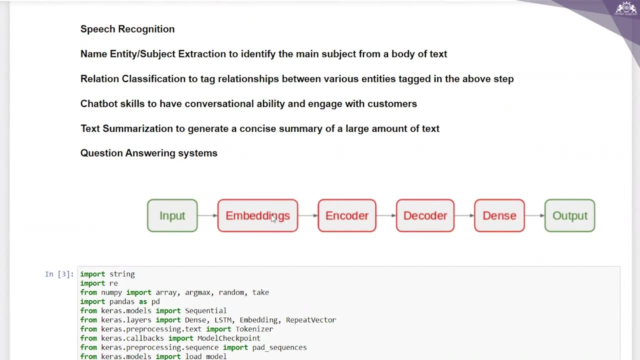 so now you can have a look at the structure. actually i have shown over here. so there is uh. for the encoder, we will be using uh embedding layer and an lstm layer, and for the decoder, i'm using another lstm layer followed by a dense layer. so here we have input embeddings. 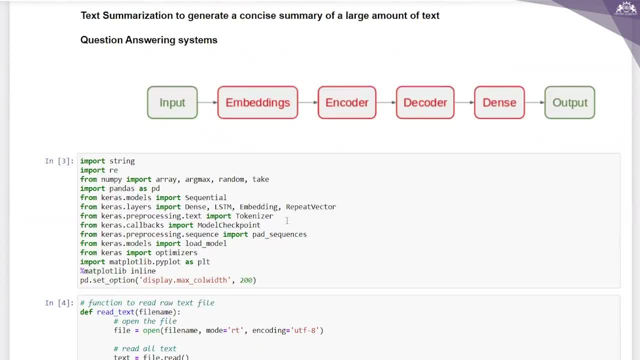 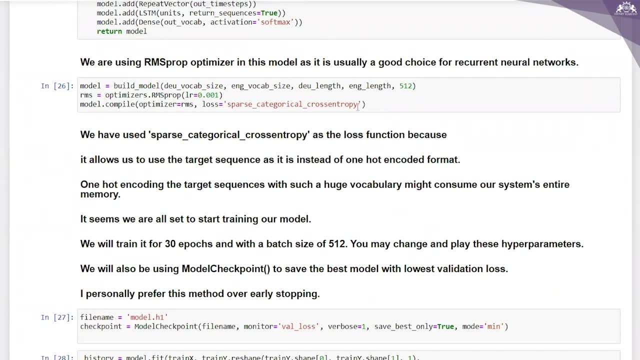 encoder, decoder, dense, and then it is being output, right. so now what i have done is what i have done is just i have used this. i have used sparse, categorical cross entropy as the last, because it allows us to use the target sequence instead of one hot encoder format. so one hot. 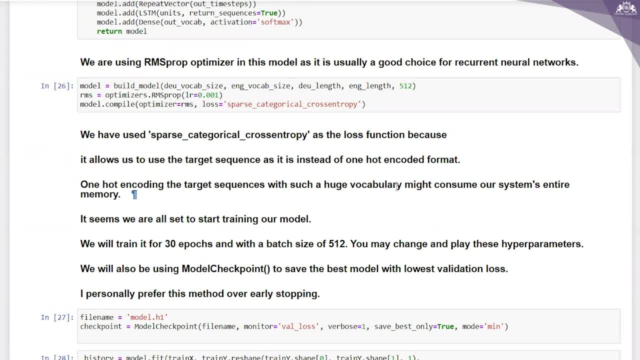 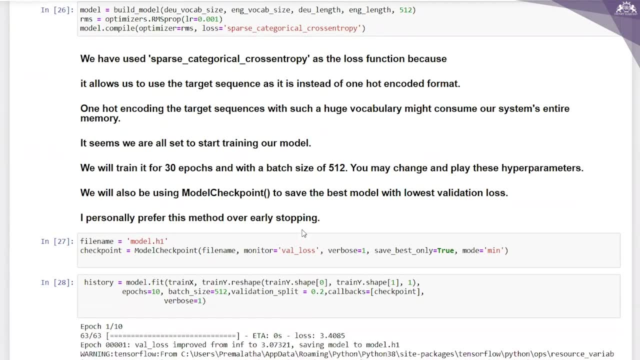 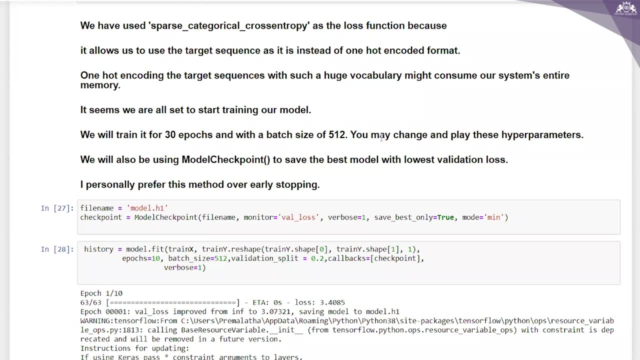 encoding uh the target sequences with the high vocabulary might consume our system's entire memory. right, so it seems we are all set to training our model. so we can try for 30 epochs, but i have taken only uh 10 epochs with a batch size of 512.. you can also change with several epochs, and 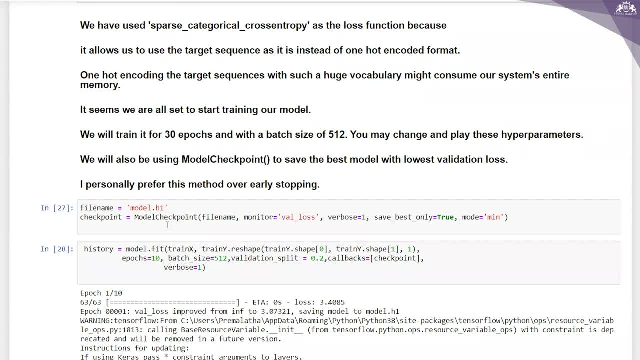 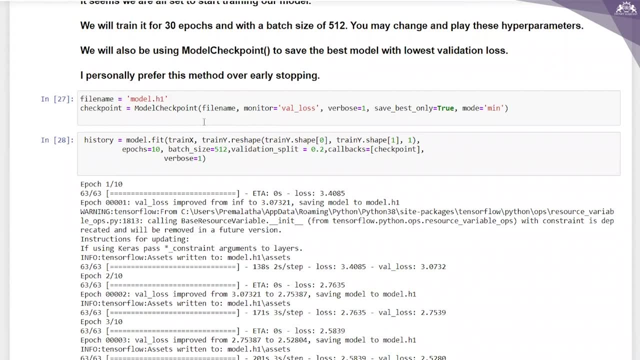 you can play with this hyperparameter parameters and also i am using model checkpoint to save the best model with the lowest validation loss right. so and also i have done this early stopping. so file name: i am saving it as modelh1 and checkpoint, model checkpoint. file name, comma. 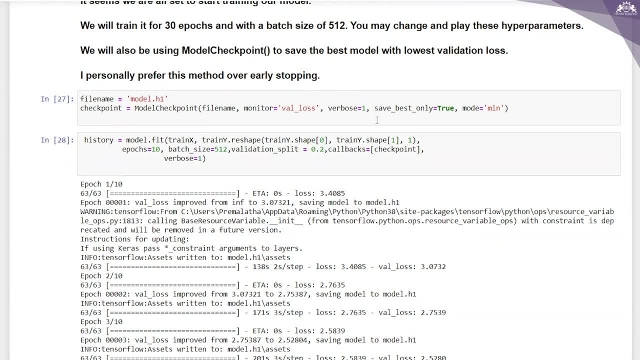 myoneter is equal to val, underscore, last and verbose, i am setting it to one. and mode is equal to minimum right. so then i'm writing: history is equal to model dot fit train x, train y, and then just i'm, i'm making the model to fit with that. so i have tried with the 10 epochs you can. 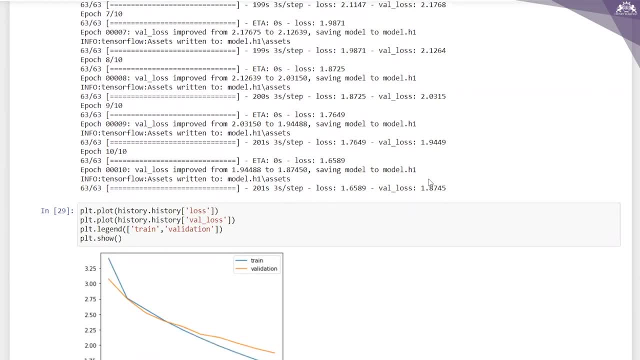 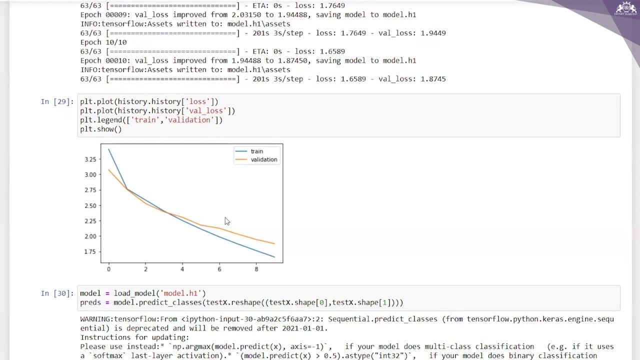 try with 20 or 30 and you can see about the validation loss and all right. so whatever is being uh, better that you can fix it up, right. so that is what we have to do, right? so once i do that, we can compare the training loss as well as the validation loss over here. so the validation loss. 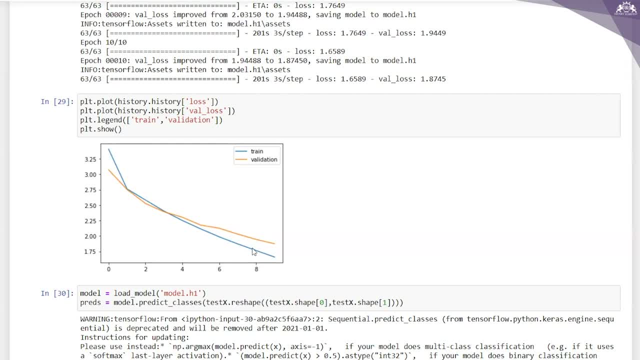 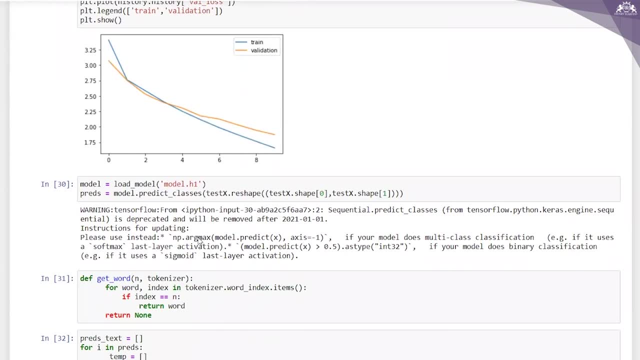 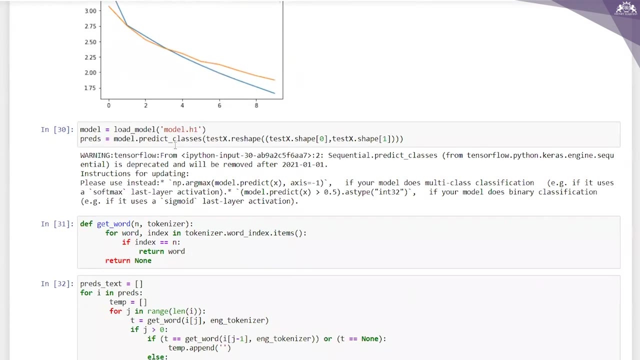 what is happening with this, that you can just look at this. what is happening to the loss over here, right? finally, we can also load the saved model and make predictions on the unseen data, that is, the test data. so what i'm doing now? um, right, so these predictions will be the sequence of the 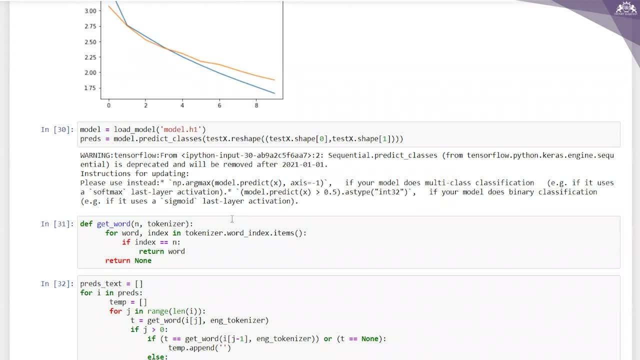 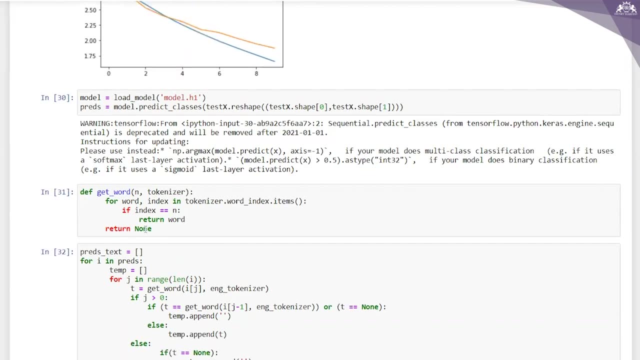 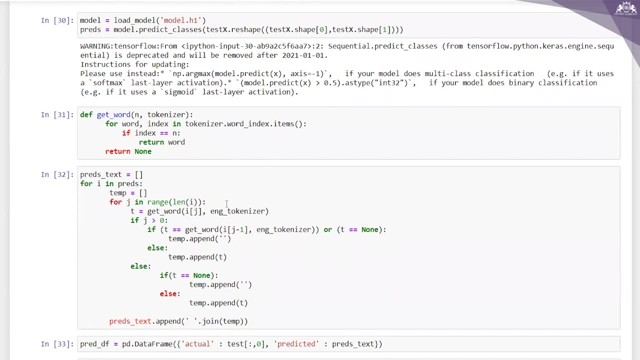 integers, so we need to convert these integers into their respective words. so that is why i'm defining a function over here: n comma tokenizer. and here what i'm doing, i'm converting the predictions into into english. actually, right, so i'm converting the predictions into english over here. and now let's put the original english. 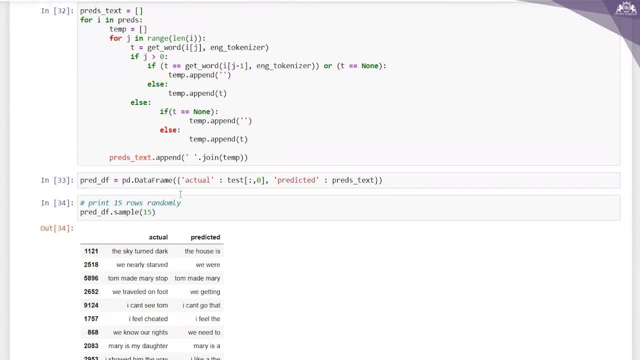 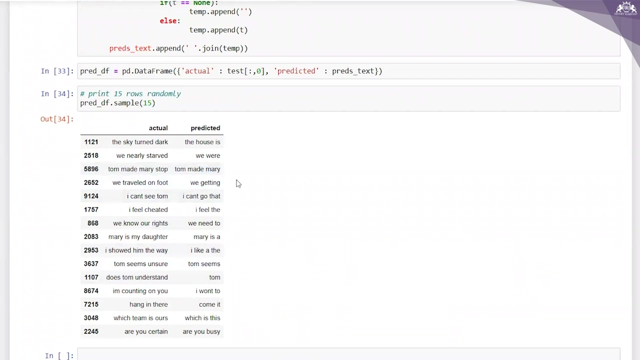 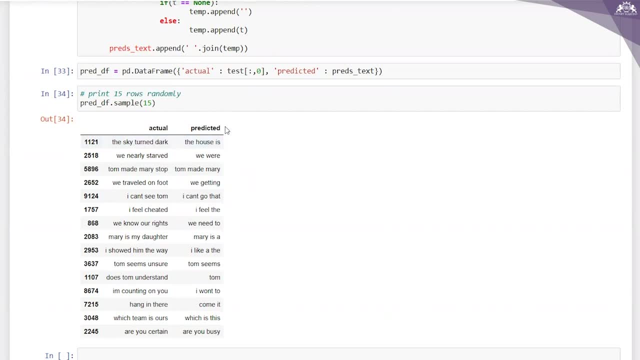 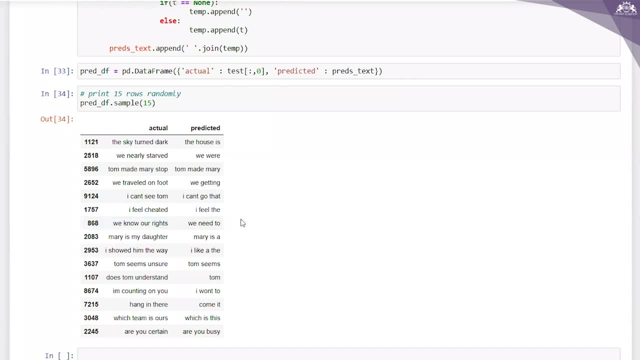 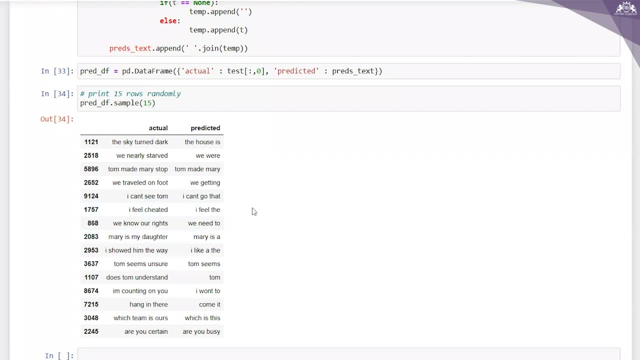 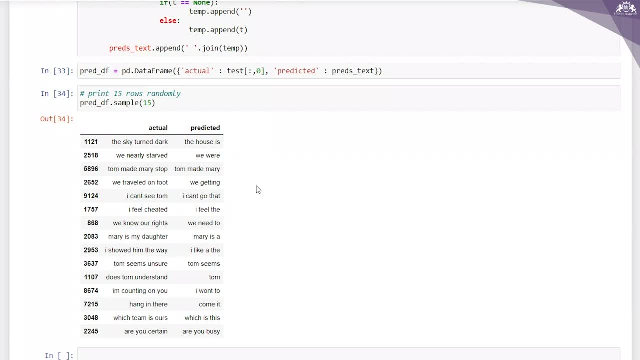 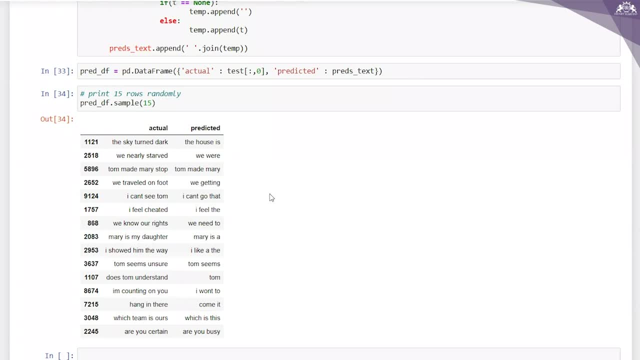 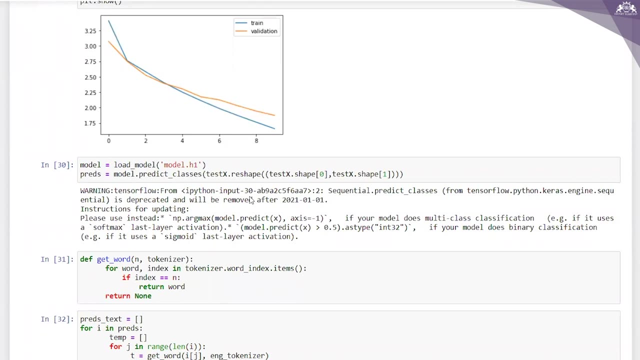 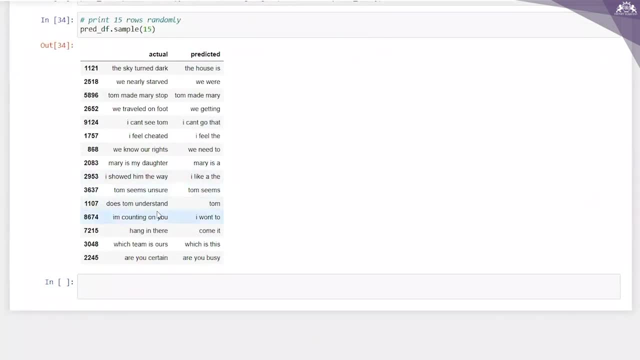 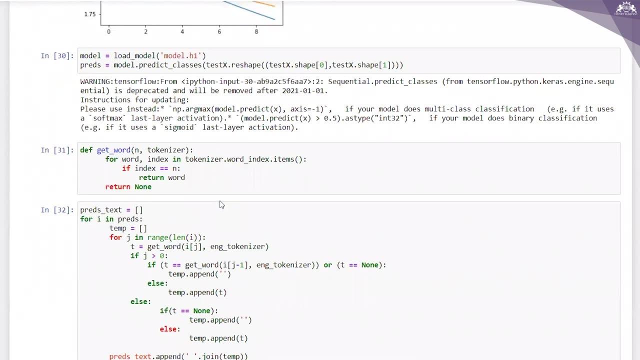 Say, I can see something like does Tom understand? So it is being stopped in, Tom and all right. So there are some misunderstanding also, misunderstanding the keywords also. So that are the challenges that we will be facing on a regular basis in NLP. 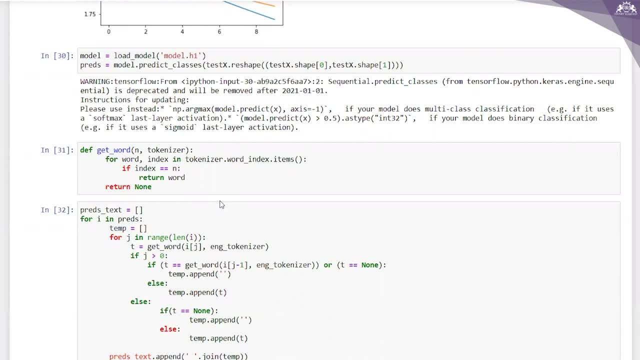 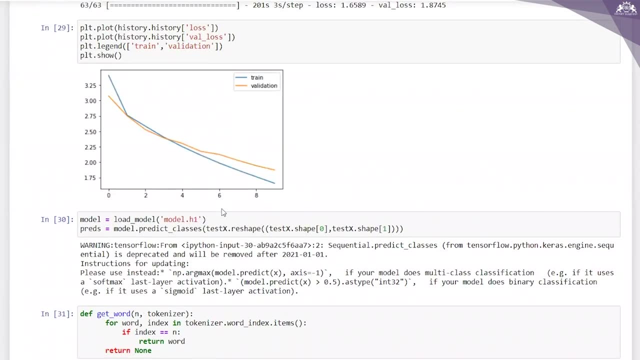 And these are not immovable obstacles. So we can mitigate such challenges by using more training data and building it better. So what I request you to do is like change the epochs to 20,, 30, or 40..